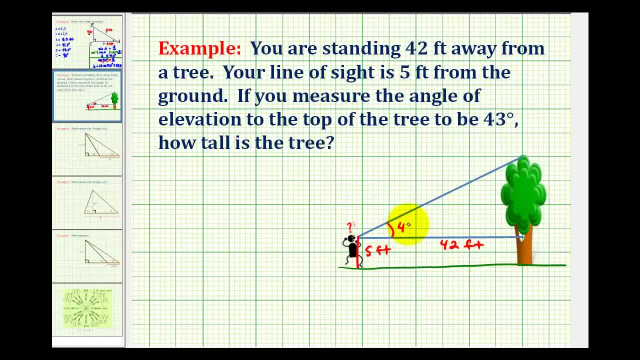 which would be the measure of this angle here, forty-three degrees. To determine the height of the tree, we'll have to do two things. We first need to determine the length of this side of a right triangle- Let's call this x- and then we'll have to add this length to the length from. 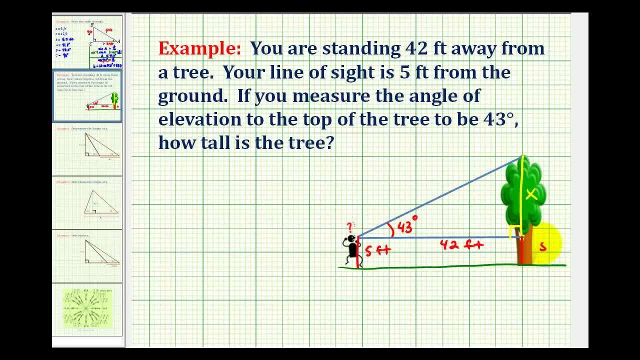 the line of sight to the ground, Which again is five feet. So if we let h equal the height of the tree, it would be x plus five. So now we can set up a trick equation to determine the length of x, Since x is the side opposite the angle that measures forty-three. 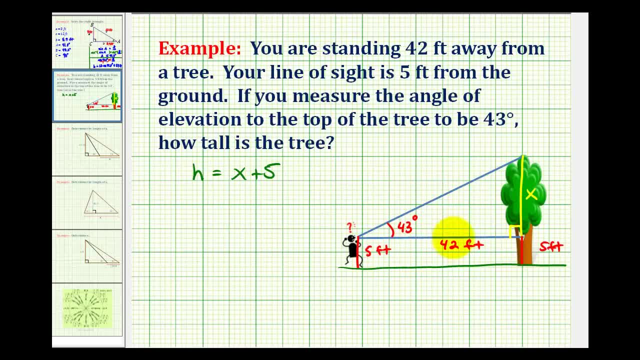 degrees, and this side here is the adjacent side. we can use a tangent function to write an equation to solve for x. The tangent of forty-three degrees must equal the ratio of the opposite side, x to forty-two. Now if we make this a proportion, we can cross multiply. 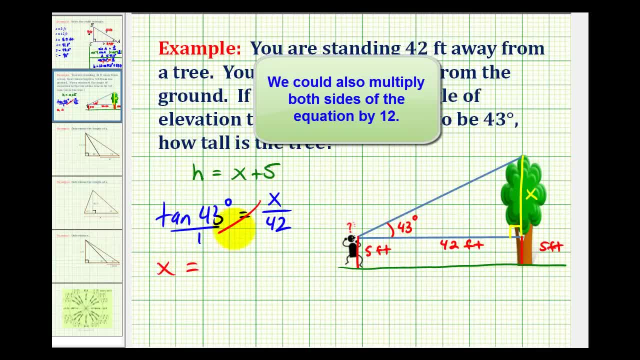 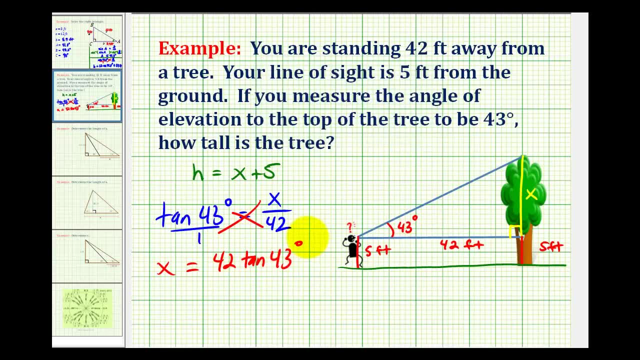 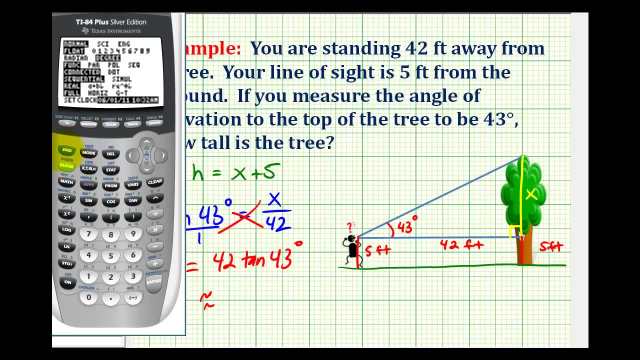 and solve for x X times one would be: x must equal forty-two times tangent forty-three degrees. And now we'll use the calculator to determine this product. Let's check our mode. We are in degree mode, So now we can just type in forty-two. 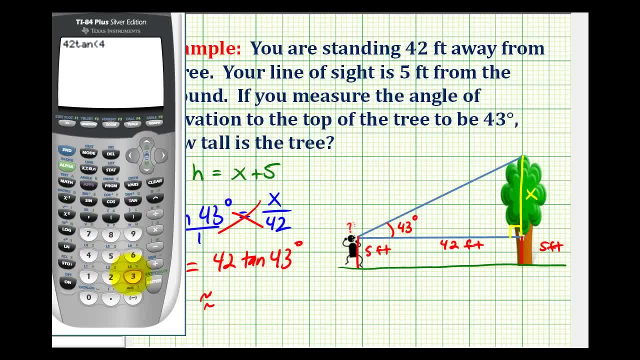 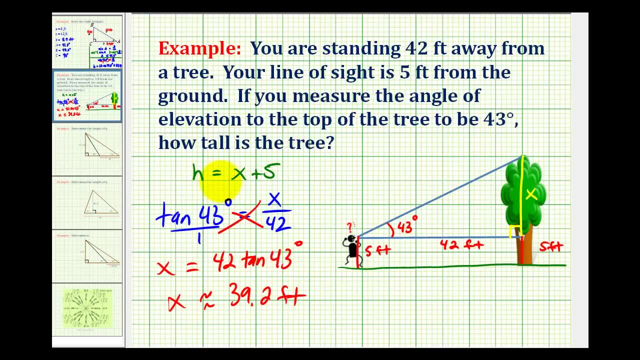 times tangent Forty-three degrees, And so x is approximately thirty-nine point two feet. But we're not quite done. Remember the height of the tree was equal to x plus five, So the height of the tree is equal to thirty-nine point two plus five. 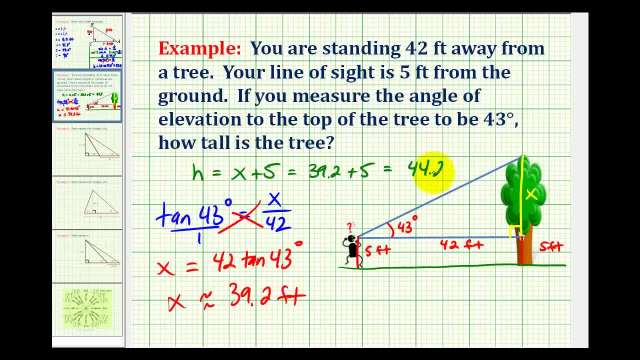 which is equal to forty-four point two feet. So the height of this tree is approximately forty-four point two feet. So the height of this tree is approximately forty-four point two feet. So the height of this tree is approximately forty-four point two feet.